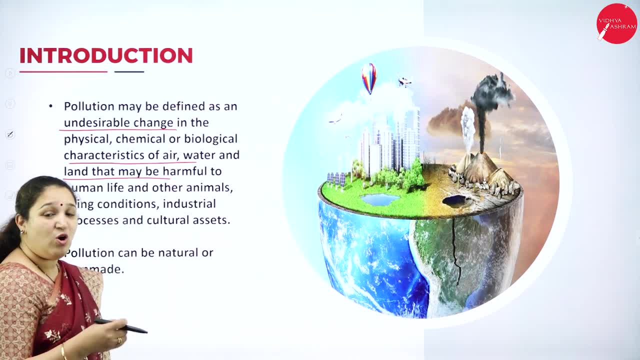 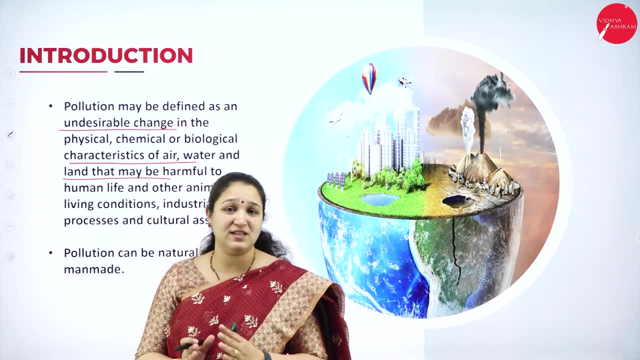 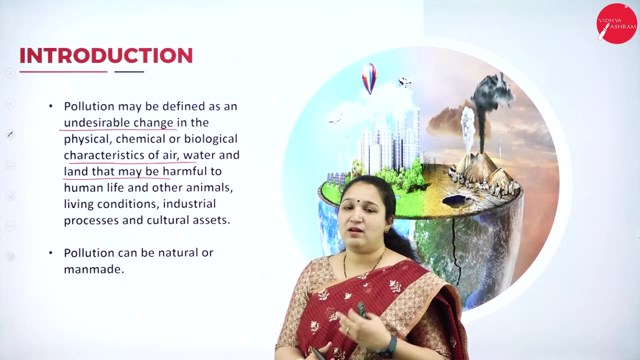 be harmful for human beings, animals or any living organisms on the earth. Okay, It's called as pollution. So any undesirable change to physical, chemical structure of water or air or land which is very harmful for any living organism and makes our life a little difficult is called as pollution. 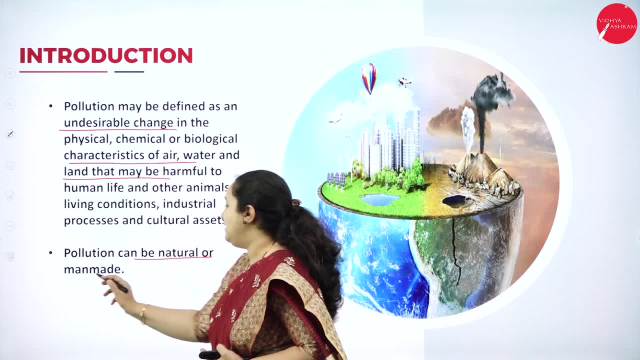 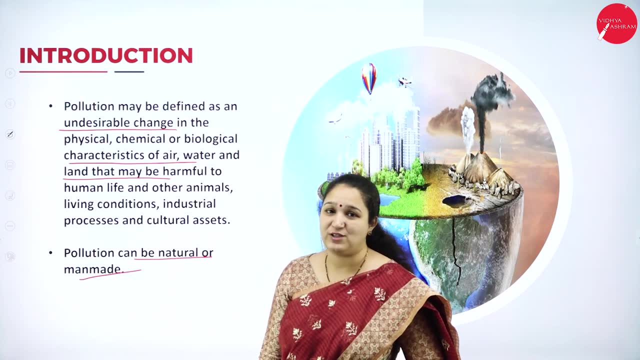 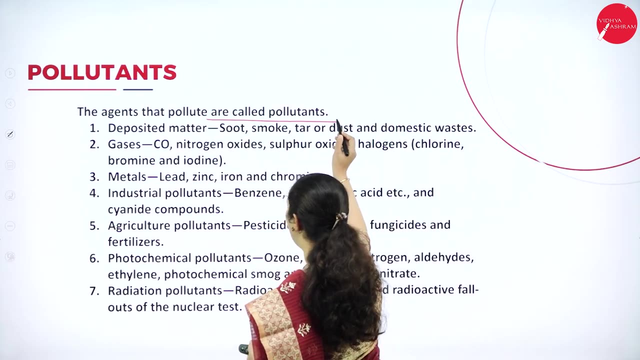 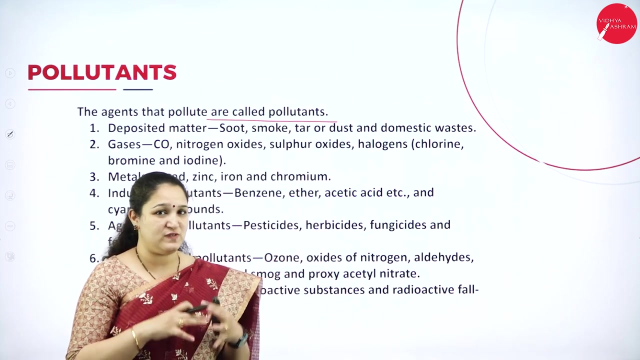 and pollution can be natural, or it can be also man-made, and most of it is man-made. then what is there natural, isn't it? So what exactly are pollutants? The agent that pollute are called as pollutants, or the extra undesirable change is brought out by addition of something that agent is called as the pollutant. 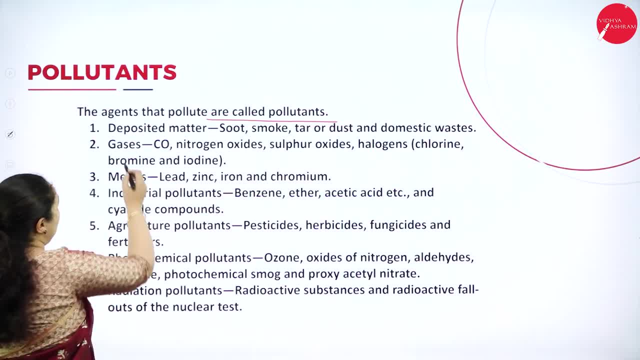 Okay, And the different types of pollutants are the deposited matter. it can be smoke, tar, dust, etc. Then it can be gases, gases like carbon monoxide, nitrogen dioxide, sulphur dioxide, sulphur trioxide, halogens containing chlorine, bromine, iodine, etc. 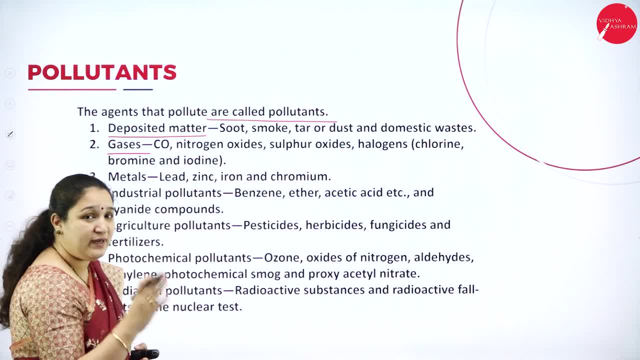 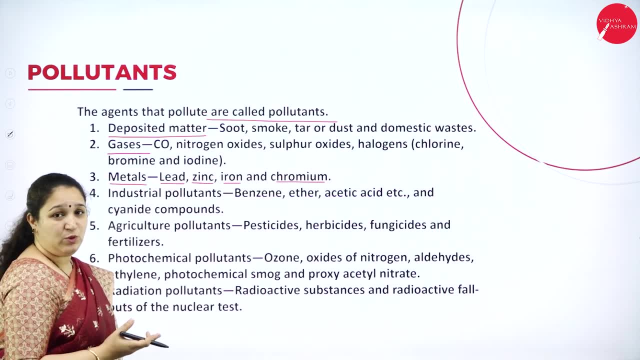 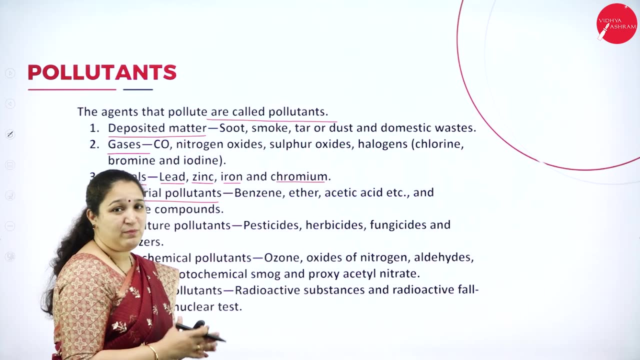 are the gases again which are acting as the pollutants. Okay, Then we can have metals like lead, zinc, iron, chromium, mercury, which are the pollutants. Then we have industrial pollutants, that is, the pollutants which are coming basically from industries that it may be in the industrial 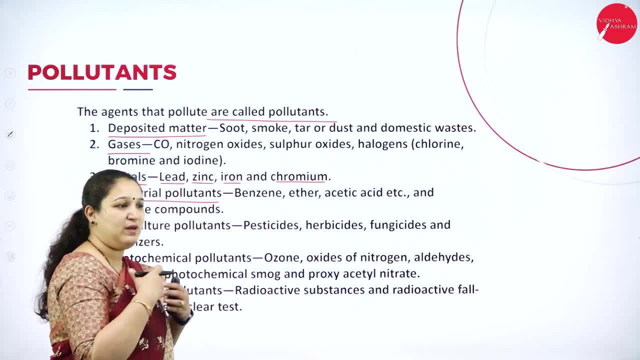 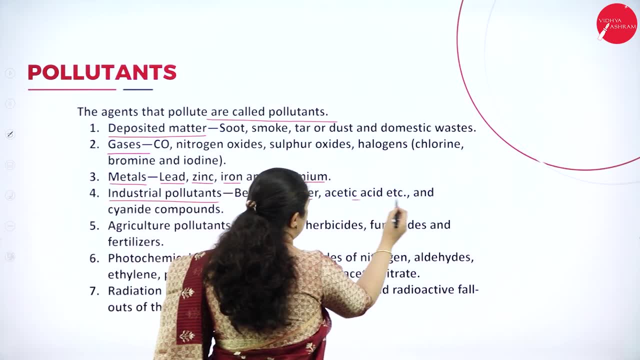 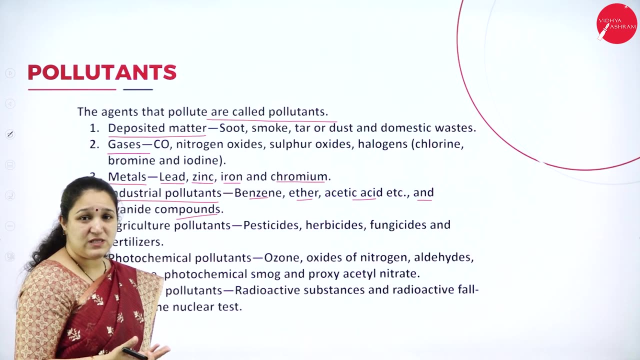 effluent, or it may be any industrial effluent byproduct. it may be the gases which are coming from the industries, etc. okay, they contain benzene, ether, acetic acid and cyanide compounds, etc. they can also have heavy metals, radioactive substances. so all of these are called as industrial pollutants. then we have agricultural pollutants. 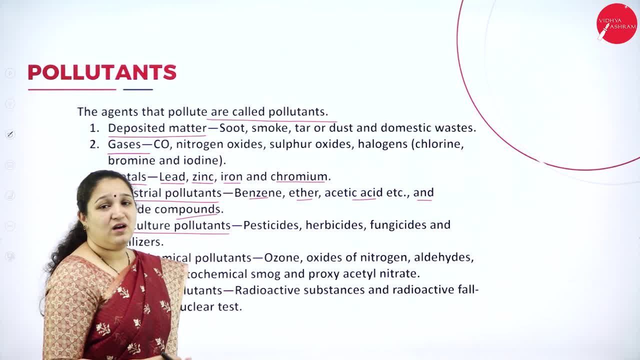 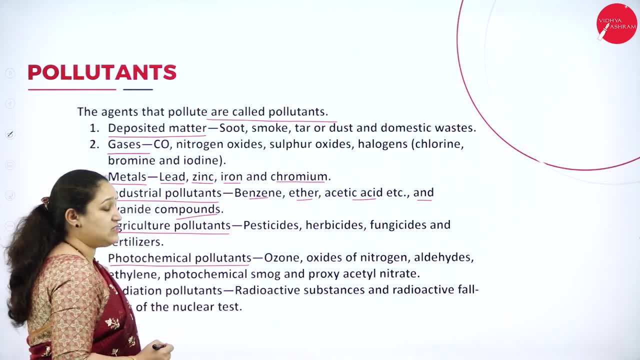 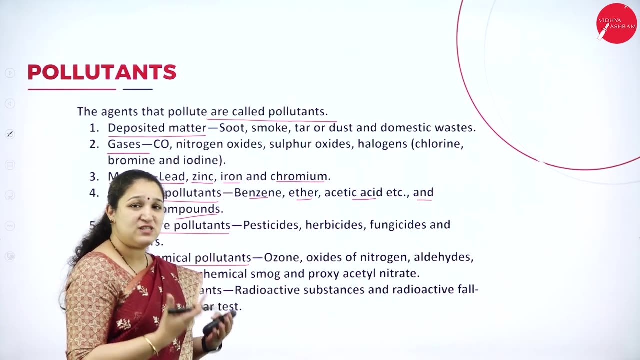 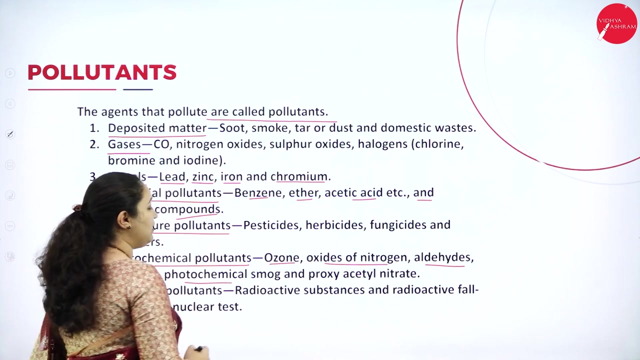 in agriculture we use pesticides, herbicides, insecticides, fertilizers, which can act as pollutants. then we have photochemical pollutants. like photochemical pollutants means these pollutants are there because of the presence of sunlight. okay, the reaction is happening because of the sunlight, so ozone, oxides of nitrogen, aldehyde. then we have ethylene photochemical. 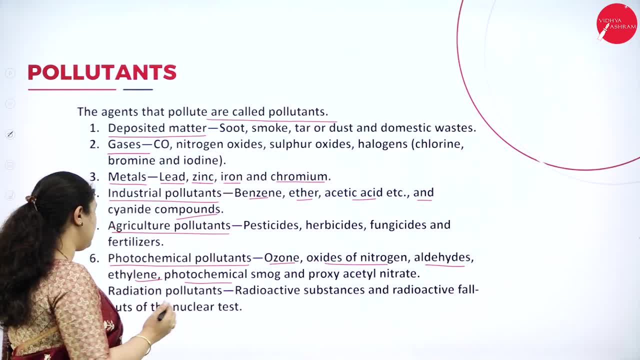 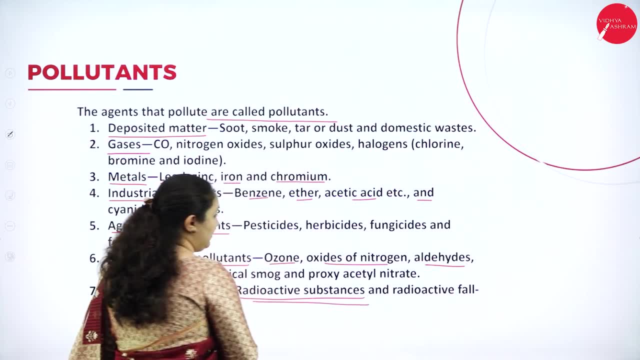 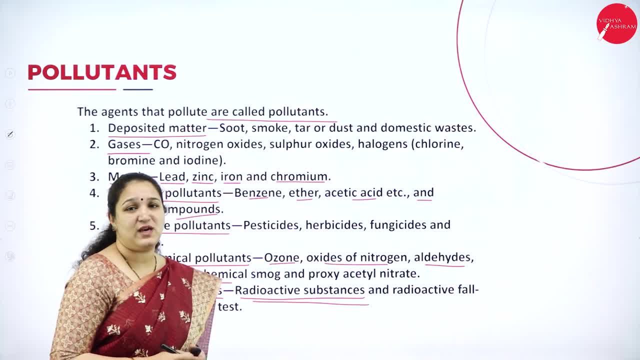 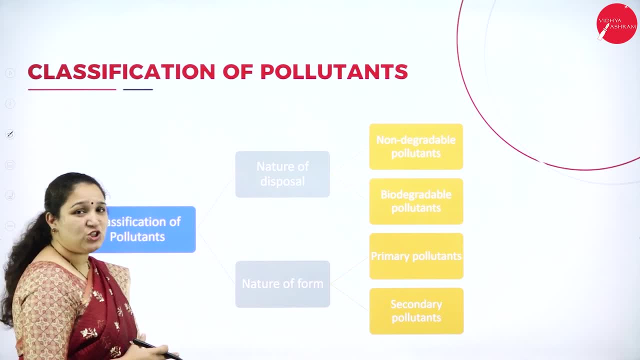 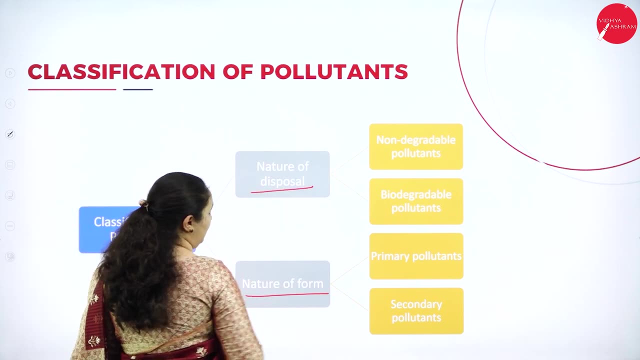 so these are basically few types of pollutants which we can see around us, isn't it? next is about the classification of pollutants. classification of pollutant, if you see it, is broadly classified as nature of disposal and on nature of how is it formed, how are we going to dispose them? 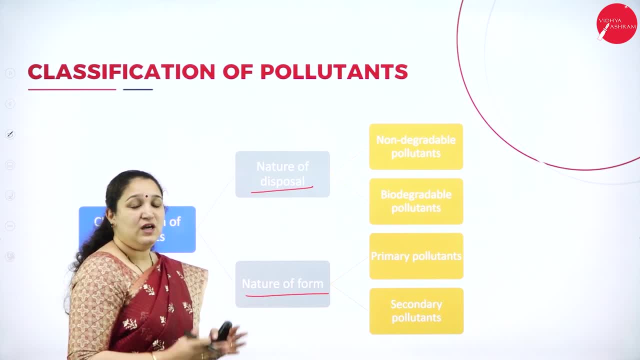 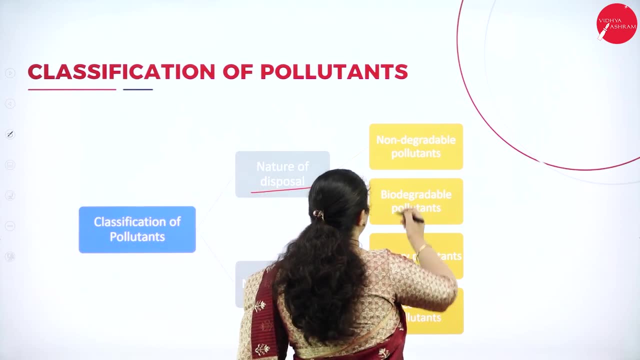 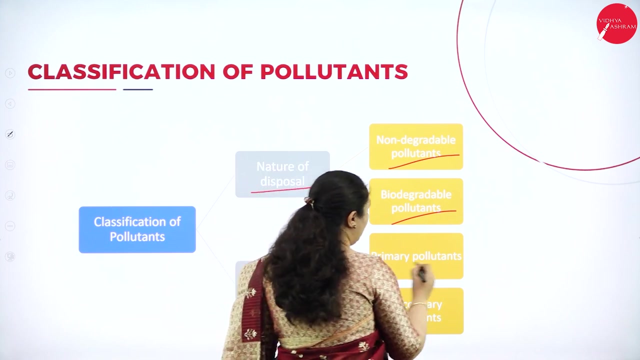 depending on that, there is one type of classification based on the у natureường. it can be non degradable or biodegradable pollutants. if it is the nature of form, we call it as primary pollutants and the secondary pollutants. okay, so we learn each one of them. 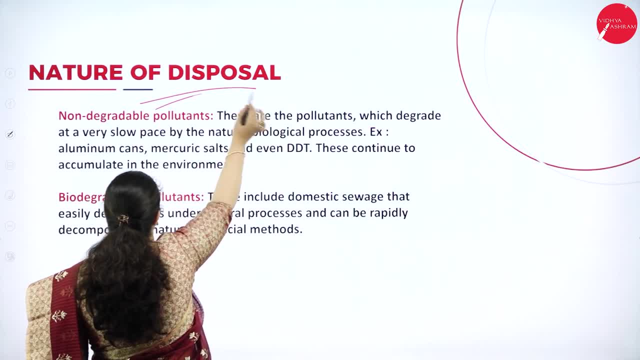 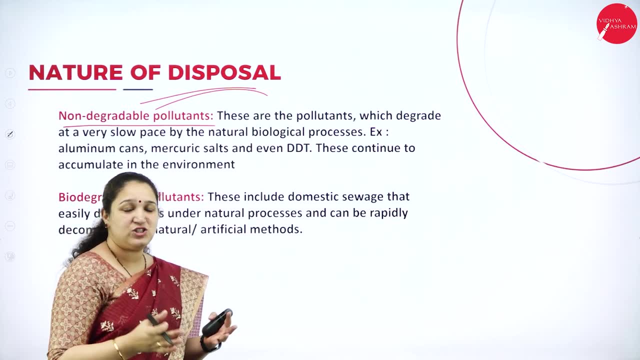 first is in itself that we followed a diesen cockey is están based on the nature of disposer non degradable pollutants. the pollutants which cannot terms of clearroduce in order cannot be degraded in the nature very easily, or it is a very, very, very slow process which 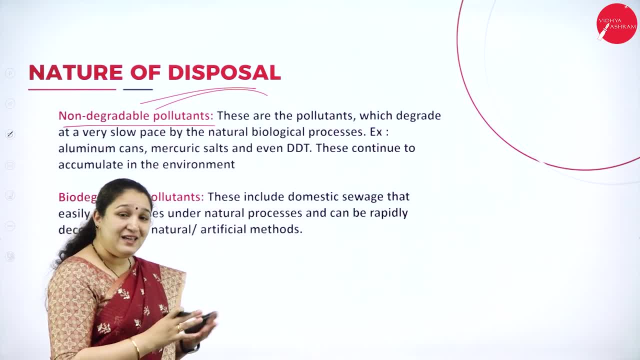 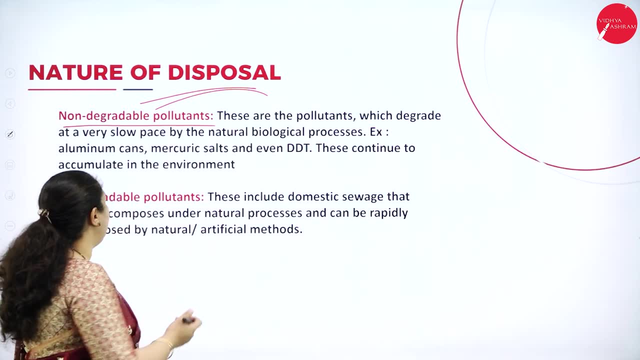 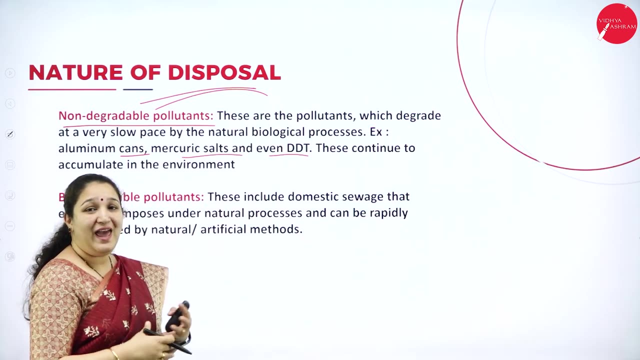 is happening? ok, no microorganisms can decompose these materials. then we call them as non degradable pollutants. example: I can give DDT or aluminium cans which we throw, anything which contain mercury, etc. they only accumulate and increase over time. ok, next is the biodegradable pollutants. 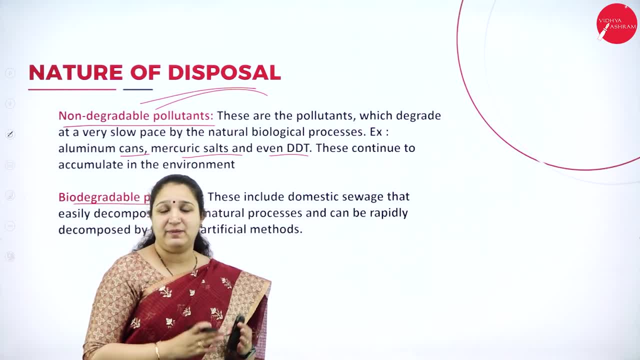 these are the pollutants which can be degraded by the microorganisms into simpler compounds. but what happens is if you accumulate the biodegradable pollutants, then the rate of accumulation is greater than the rate of decomposition and this can create a lot of problem in composting. 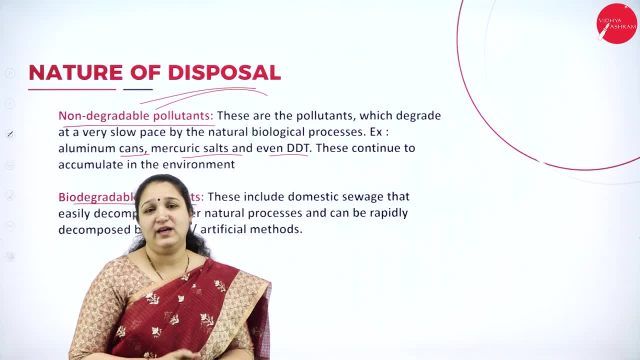 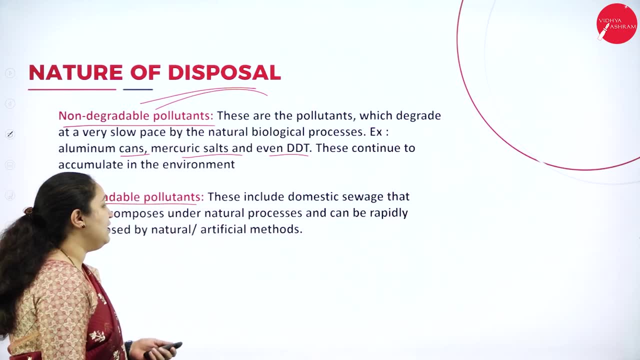 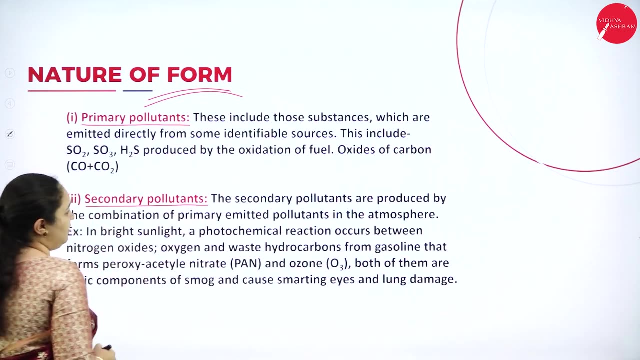 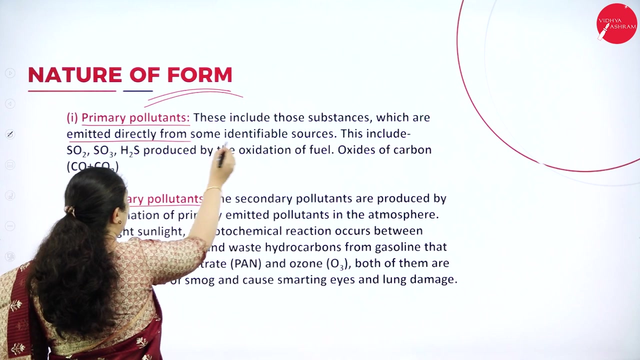 Next, we have соответ, two limits of polluter pollution. okay, othersассlogo. So here we have two perspectives. the primary pollutants which are causing pollution, ok. example for Biodegradable Pollutants are: we can take domestic sewage. they are biodegradable pollutants, ok. next, we have based on the nature of form. 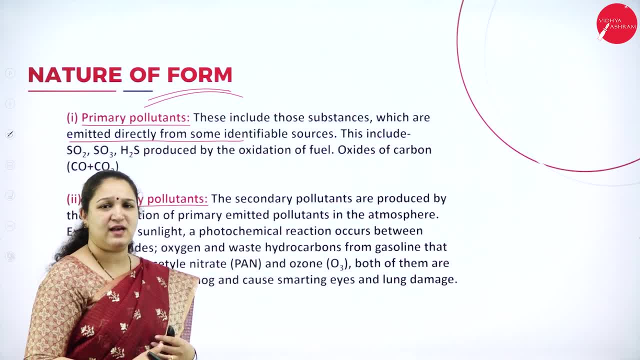 it is primary pollutants and the secondary pollutants. primary pollutants: these include those substance which are emitted directly from a particular source, For example from industries, directly from a particular course. When I have these disposable or disposable organic contaminants of the form above them, we are getting nitrogen dioxide gas, sulfur dioxide gas, carbon monoxide gas, hydrocarbons, etc. 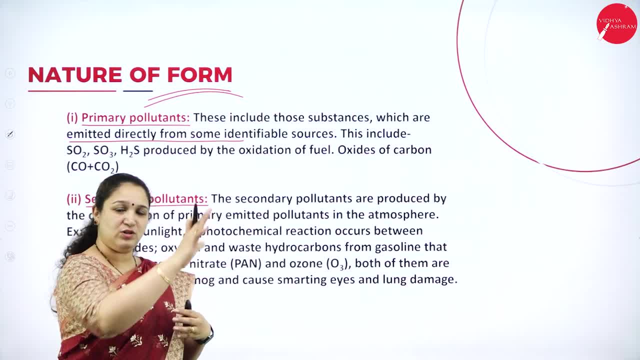 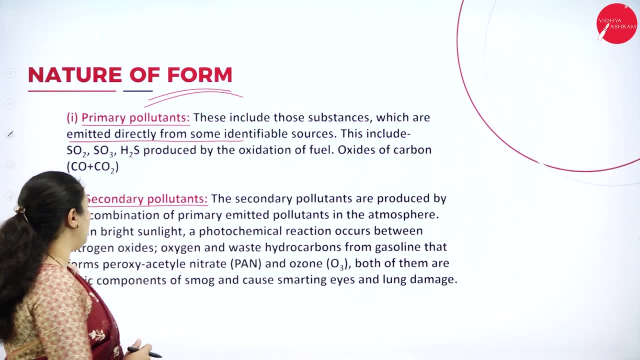 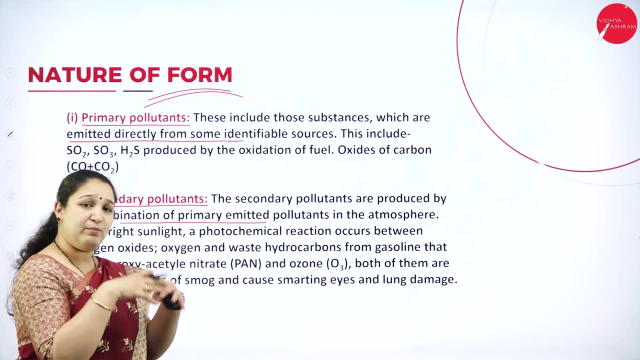 these are directly which is there. it is directly coming into the environment from the source. then it is a primary pollutant, secondary pollutant. the secondary pollutants are produced by combination of primary emitted pollutants in the atmosphere. so the primary pollutants which are coming they combine with one another to form one more pollutant. we call it as a secondary pollutant. 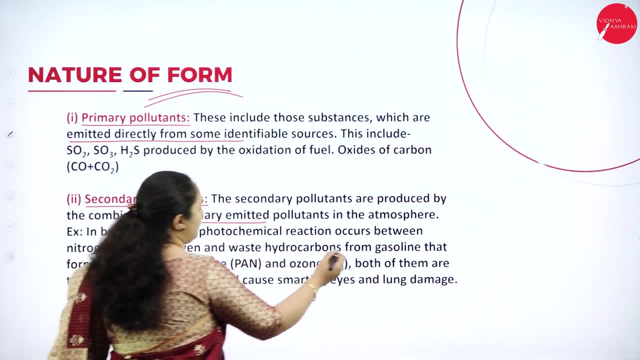 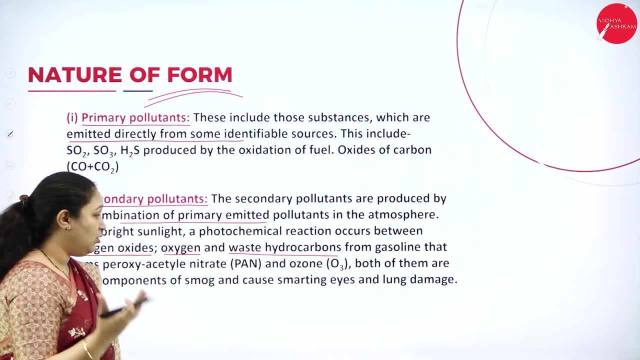 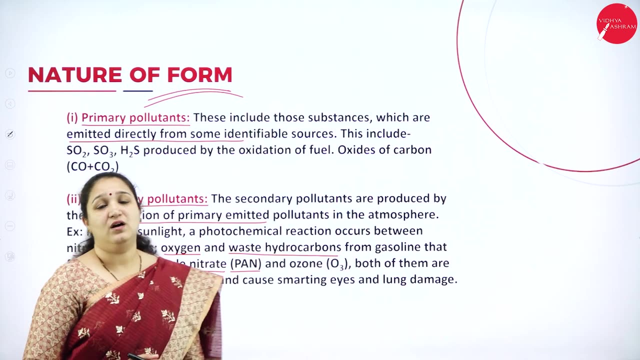 example we can give in bright sunlight. photochemical reaction occurs between nitrogen dioxide and oxygen and waste hydrocarbons to form, you know, per oxy, acetylene nitrate, that is, pan, and ozone, which is a secondary pollutant. okay, next is about different types of pollution. 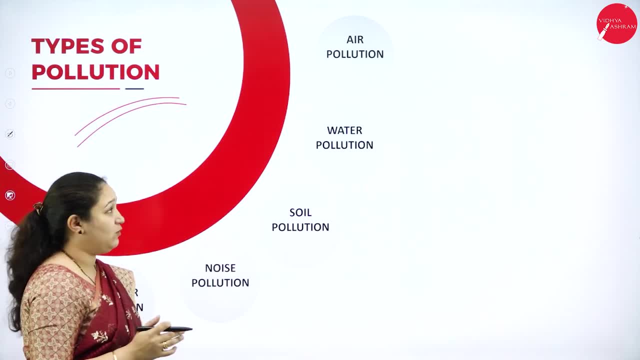 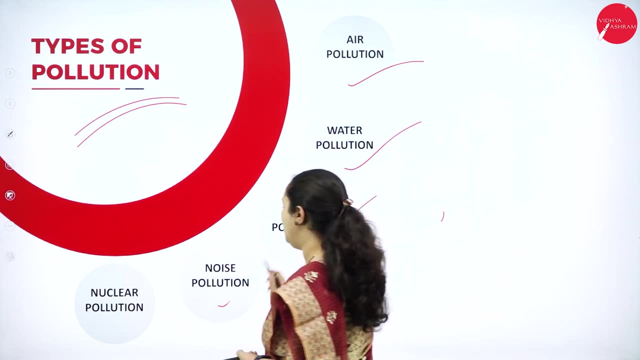 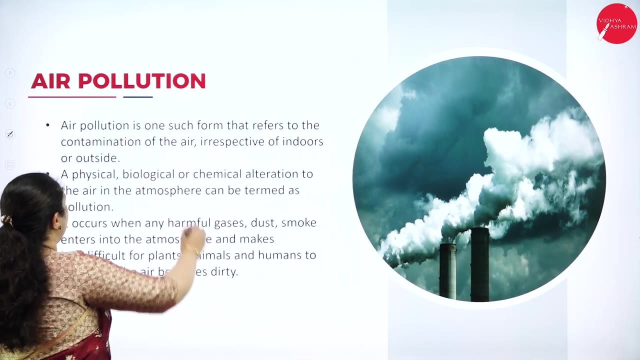 which we are going to study in this particular chapter. okay, we will study about the air pollution pollution, water pollution, soil pollution, about the noise pollution as well as the nuclear pollution. So first we will go into the details of air pollution. What is air pollution? Air? 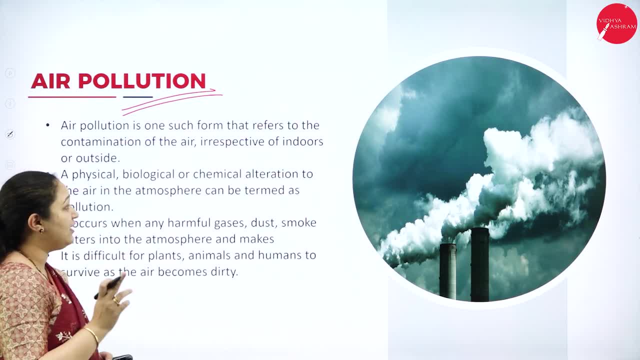 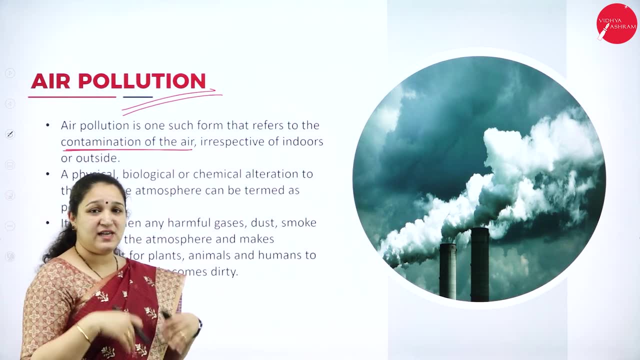 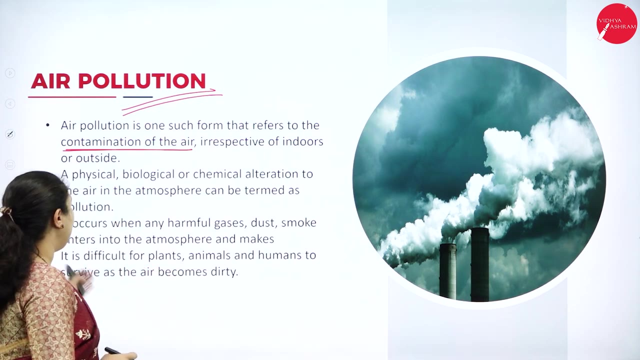 pollution is one such form. that refers to the contamination of the air, irrespective of indoor or outdoor, Whether it is inside or whether it is outside environment. totally, if the air is getting contaminated, we call it as air pollution. Then we have a physical, biological or chemical 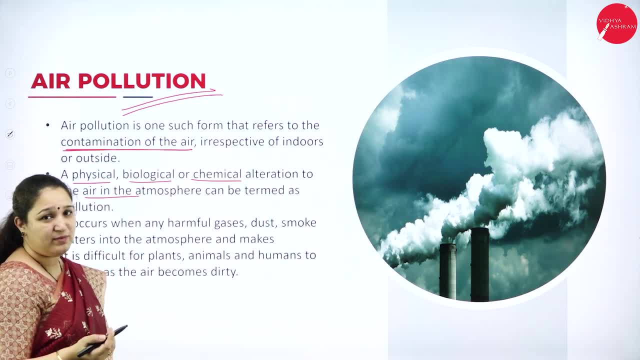 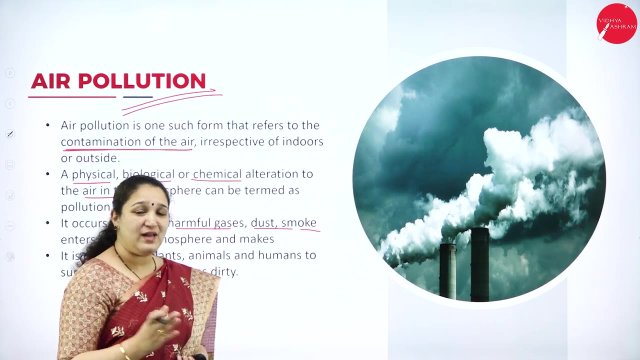 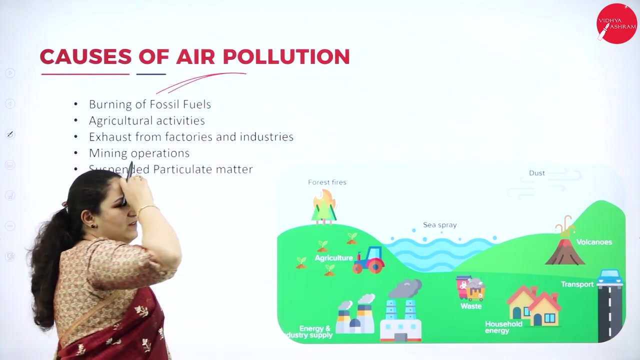 alteration to the air in the atmosphere is also termed as air pollution, and it occurs when there is harmful gases. dust, smoke enters into the atmosphere and makes our life difficult because there is dirty air around us, So that is called air pollution. Next is about the causes of air pollution. There are several causes of air pollution which we can. 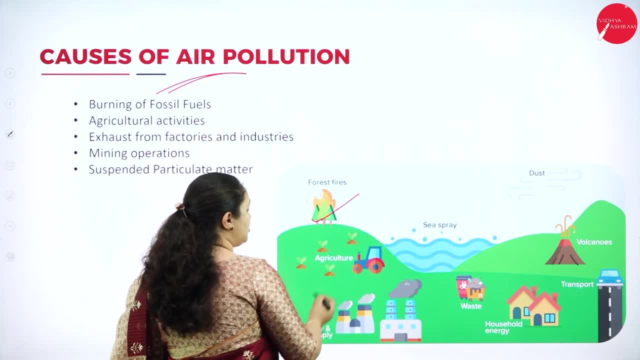 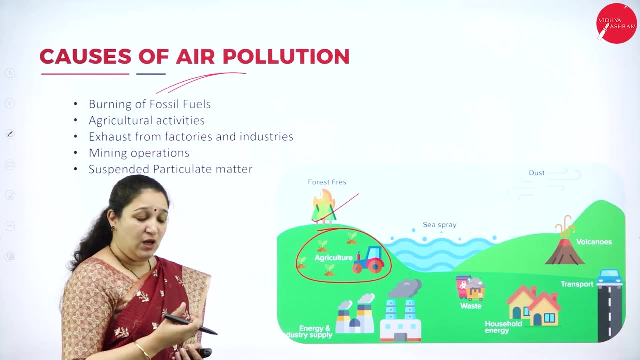 see, For example, forest fires causes air pollution. agriculture causes air pollution. You might ask me how agriculture is causing air pollution, ma'am, That is when there is spraying of pesticides or insecticides, which we are doing, those aerosols go into the air and that causes pollution. 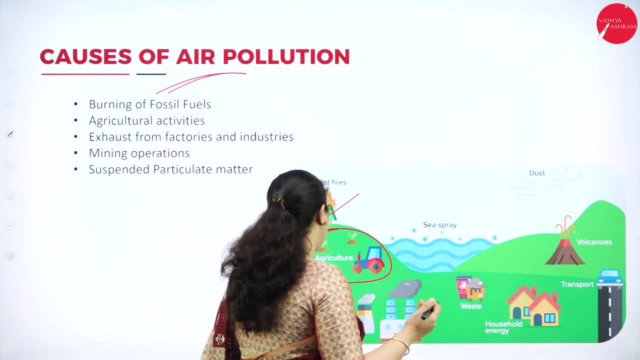 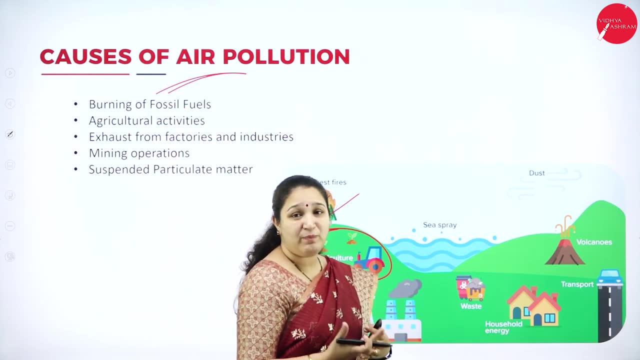 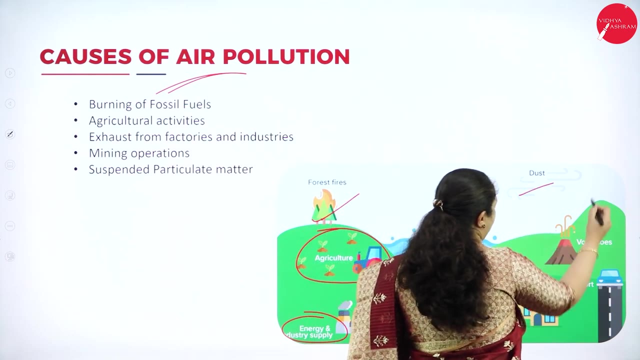 So even agriculture can cause pollution. Then we have energy and industry supplies, that is, from the energies and industries as well. as there are nuclear power plants where the energy is produced, Okay, There also air pollution can happen. Then there is a lot of dust, volcanoes, transport, household energy from the waste- All of this there is a lot of. 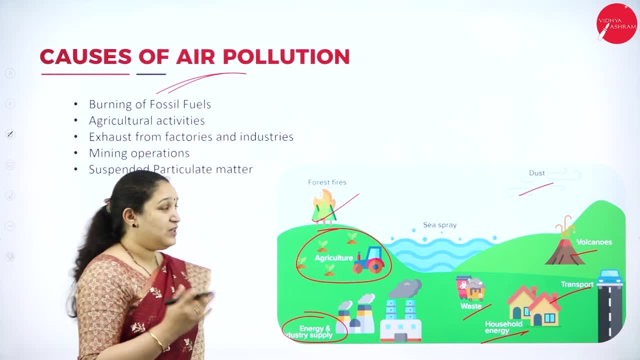 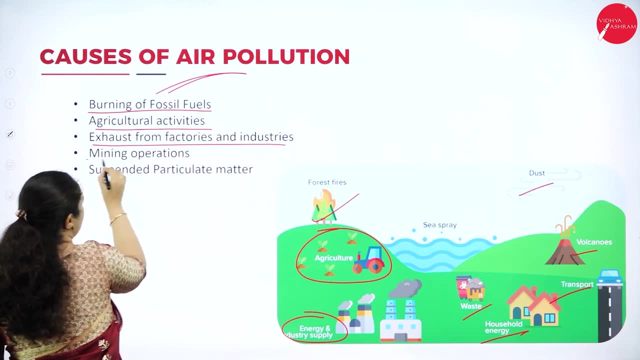 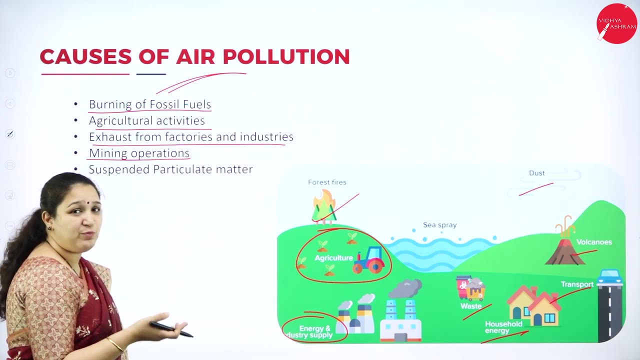 pollutants which is coming out, which causes air pollution. So we have burning of fossil fuels, agricultural activities Exhaust from factories and industries, mining operations- we have already studied of effects of mining operation under that. air pollution also was there, isn't it? 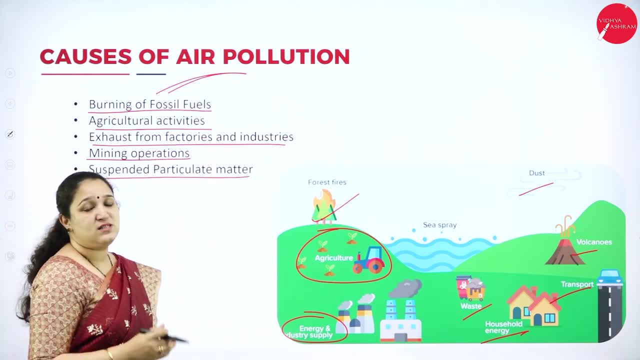 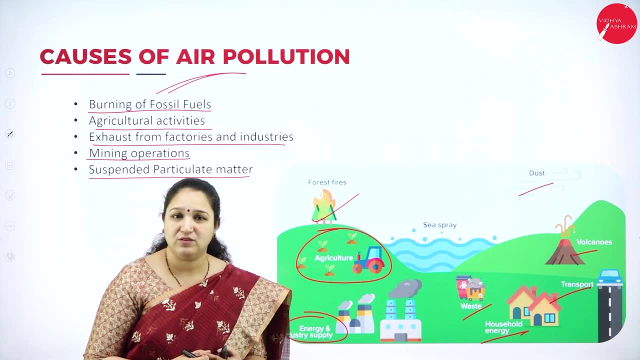 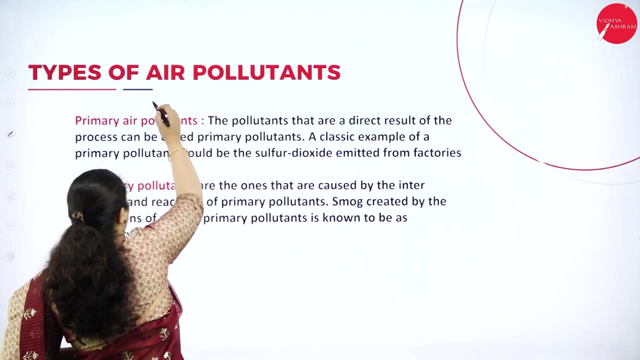 Then we have suspended particulate matter, that is, we have lot of fog which is formed because of the other air pollutants are few of the causes of air pollution. Next is about the different types of air pollutants. We have primary and secondary, as I explained. 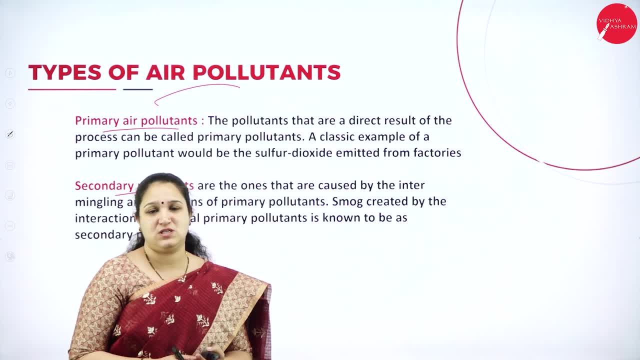 Primary air pollutants is from the primary source. it is coming. Example: I gave you different gases like sulphur dioxide, carbon monoxide, etc. And secondary pollutants are those which is caused by the reaction of the primary pollutants. So primary pollutants will react to give rise to secondary pollutants. 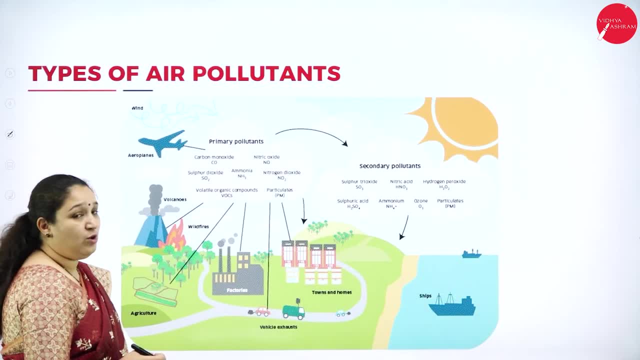 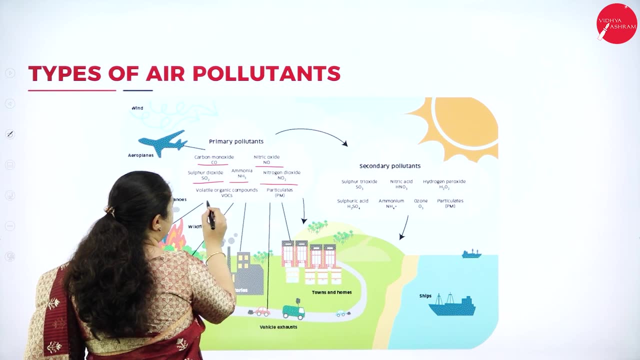 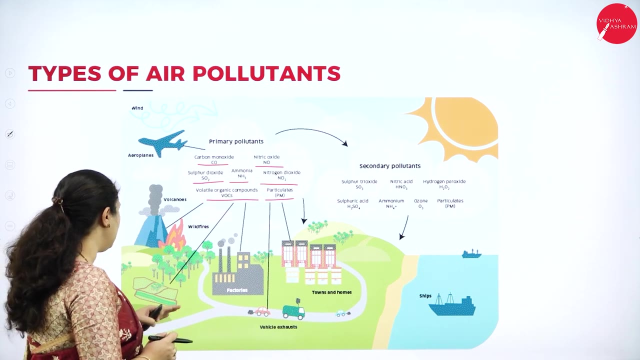 So we can see here some of the primary pollutants which we have: Carbon monoxide, nitric oxide, sulphur dioxide, Ammonia, nitrogen dioxide, volatile organic compounds and particulates which is there. All of this is directly coming from volcanoes. you know agriculture or forest fire factories. 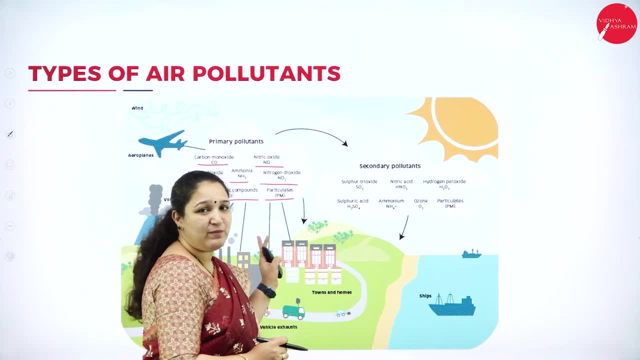 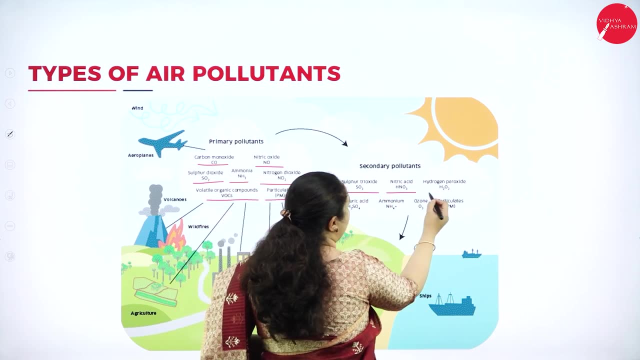 from the vehicles or towns and homes. We have all the primary pollutants, which we are coming Secondary pollutants. these pollutants give rise to this, that is, sulphur trioxide, nitric acid, hydrogen peroxide, sulphuric acid, ammonia ozone. 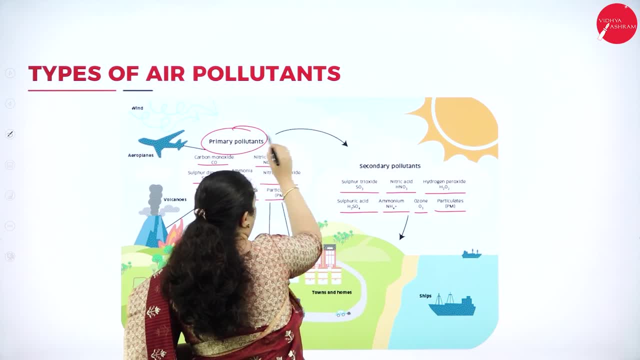 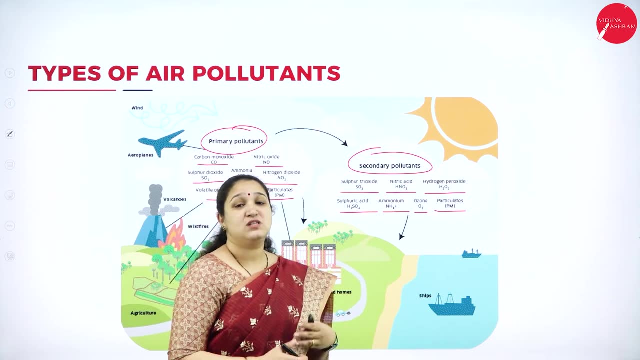 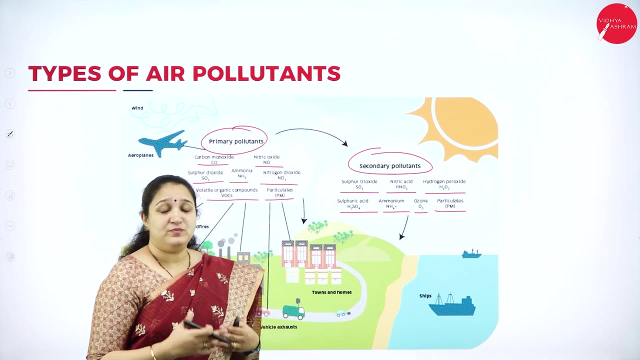 Particulate matter. is these reacted to give rise to the secondary pollutants which again will come back to the earth's surface and cause different effects, like acid rain, ok, And they will spoil our crops also. you know, lot of ailments can come up in humans, like 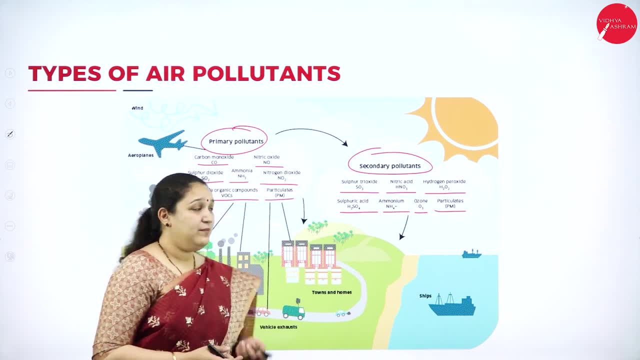 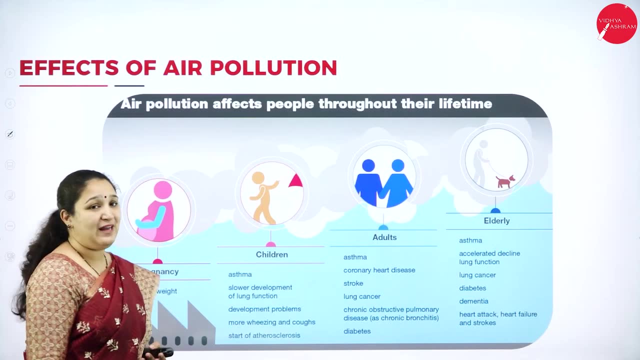 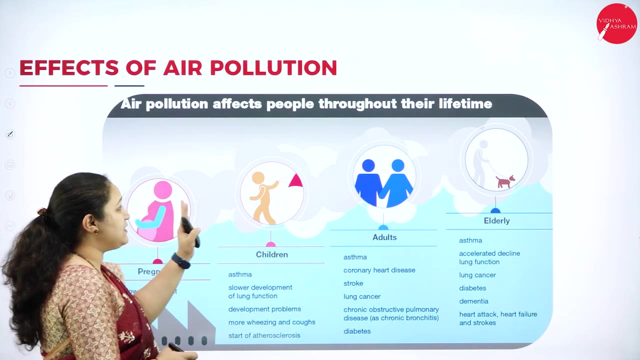 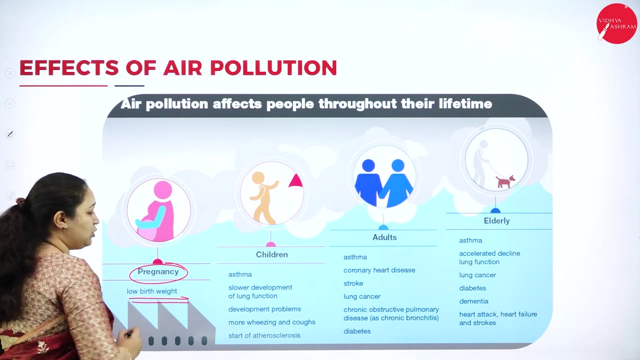 asthma or cancer, etc. Ok, So that is about the types of air pollutants. Next is about the effect of air pollution. First is the effect of air pollution on humans, which we can see. Air pollution affects people throughout their lifetime. You can see here. during pregnancy it can cause low birth weight. that is the child which is. 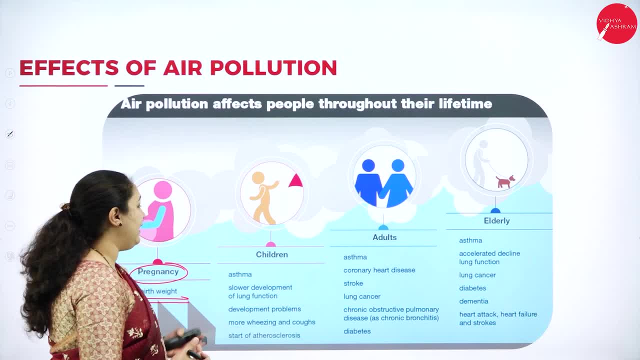 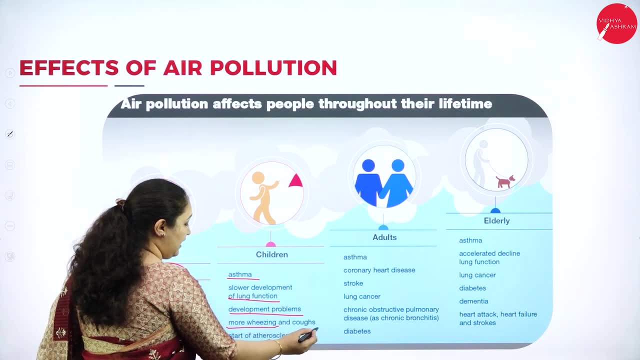 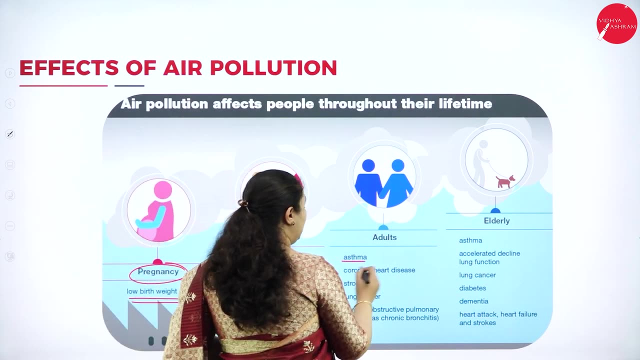 going to be born can have a low birth weight And in children it can cause asthma, slower development of lung function, developmental problems When they start sneezing and cough start. atherosclerosis. also can happen in children, In adults again, asthma, heart disease, stroke, lung cancer, chronic obstructive pulmonary. 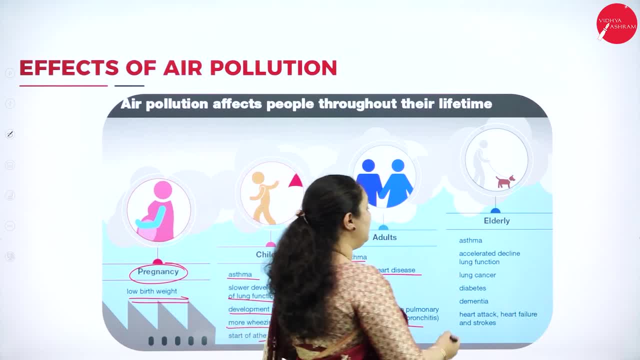 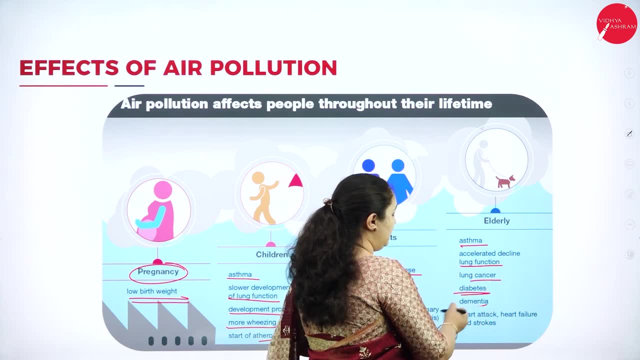 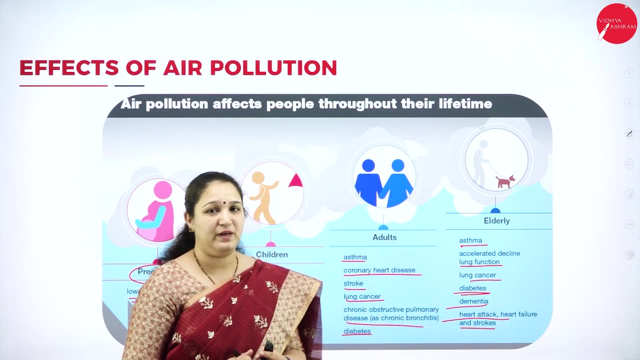 disease, diabetes etc. And in elderly again, asthma, lung accelerated decline in lung function. then you can see lung cancer, diabetes, dementia, heart attack, heart failure and stroke. All of these problems. The root cause can be Air pollution or the pollutants which is there. 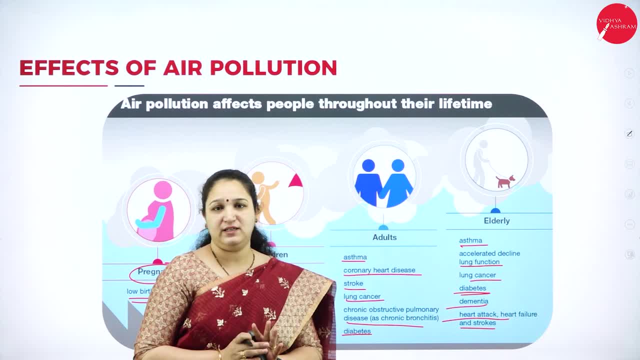 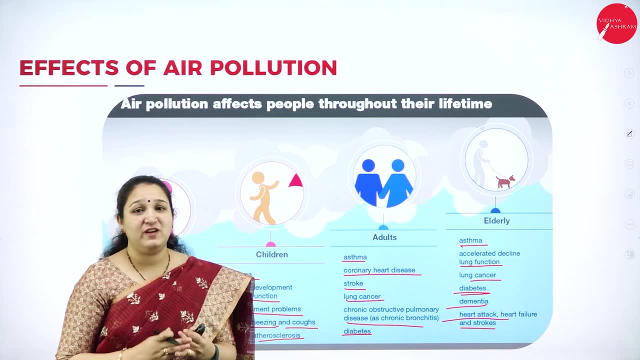 Asthma. you can see it is there in children, adults as well as elderly. That is basically because the air which we are breathing is going into the lungs, which can cause asthma, wheezing or lung cancer and along with that there are other diseases. 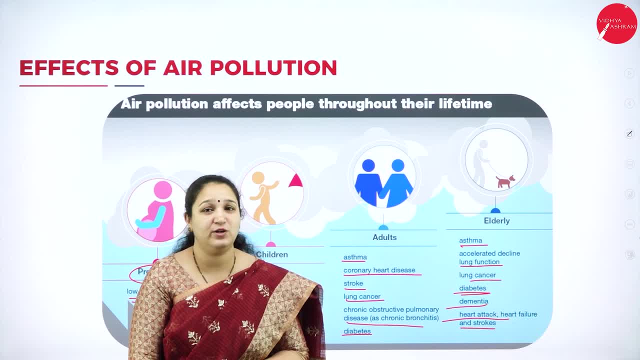 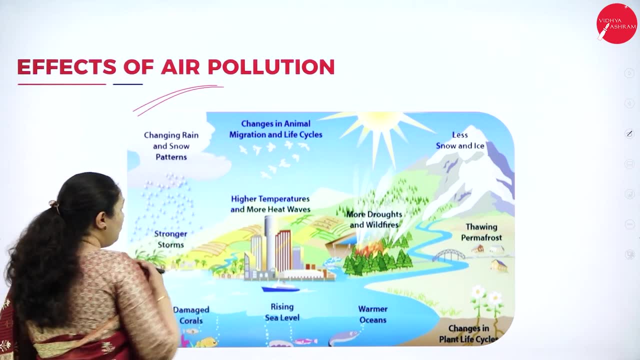 which is coming hand in hand, which can be caused basically due to air pollution. Ok, If we see the effects of air pollution, What is air pollution? What is air pollution? The other effects other than the effect on humans? we can see the changing rain and snow. 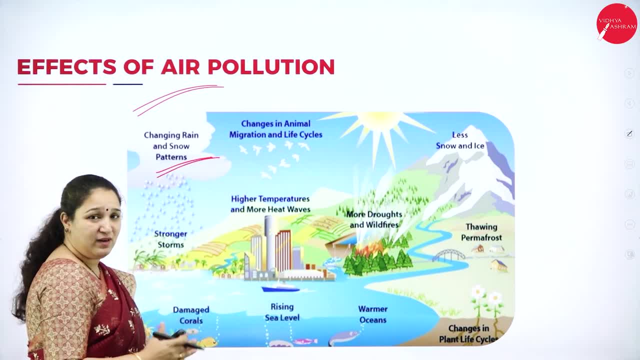 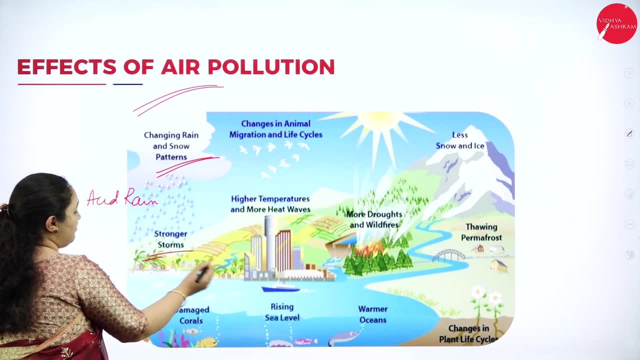 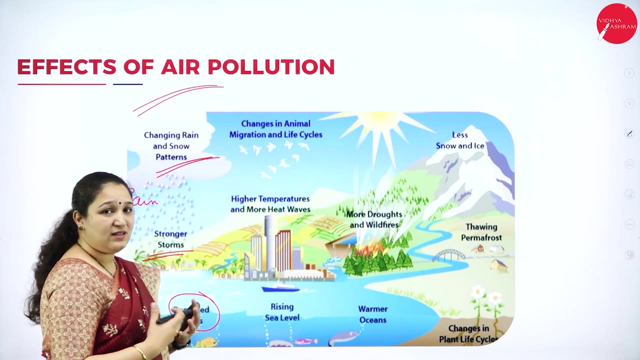 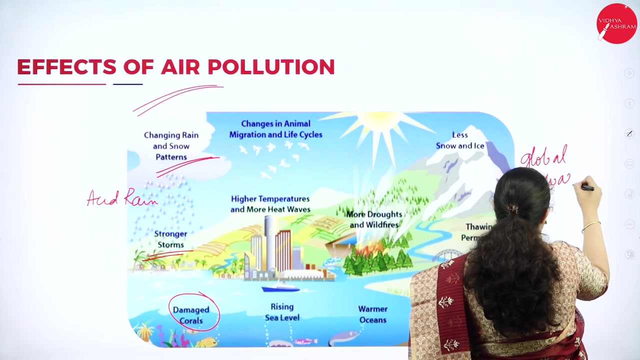 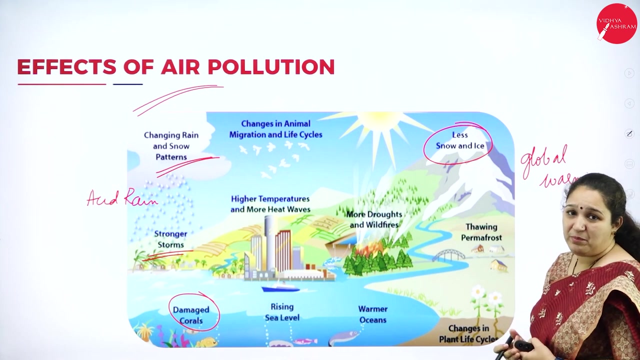 patterns: ok, and the rain pH can reduce to cause acid rain: ok. There can be stronger storms. The acid rain can damage the corals. Now, the carbon dioxide and other gases can increase global warming- Ok, And the global warming starts increasing the temperature of the earth as well as the glaciers. 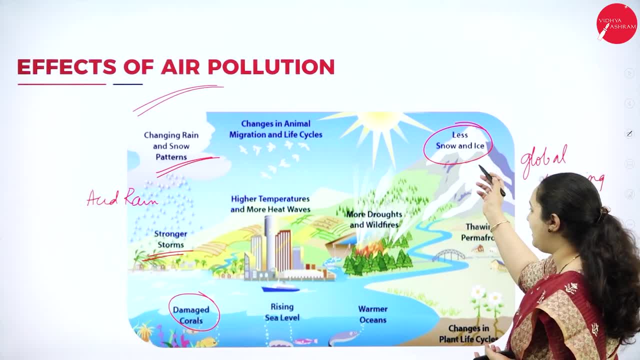 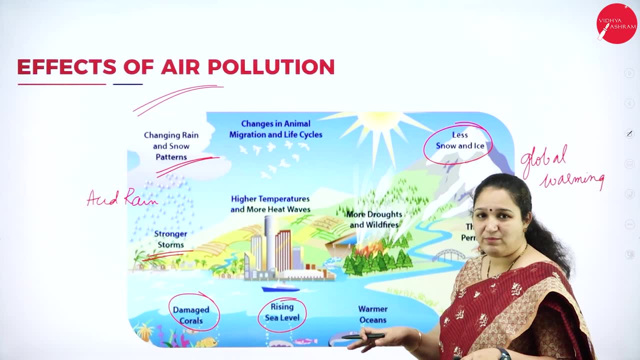 and the snow start can start melting. so less snow and ice, which gives rise to rising sea level. Rising sea level means the land is getting submerged. We have very little amount of land for the population. what we have that is very, very less what we have- land. 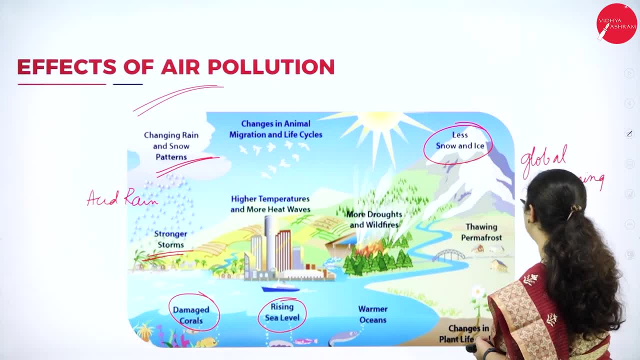 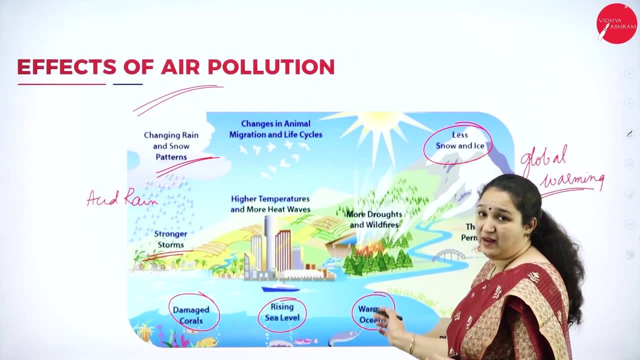 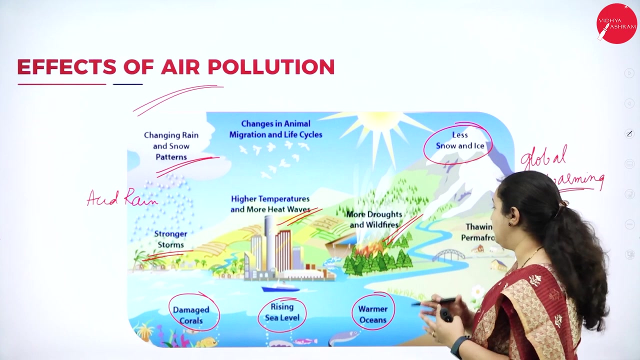 And that also starts submerging because of, again, air pollution or global warming. Then we have the temperature increases also. we will have warmer oceans, higher temperature and more heat waves will be there because of global warming. again, More droughts and wild fires or the forest fires are there because of the increased temperature. 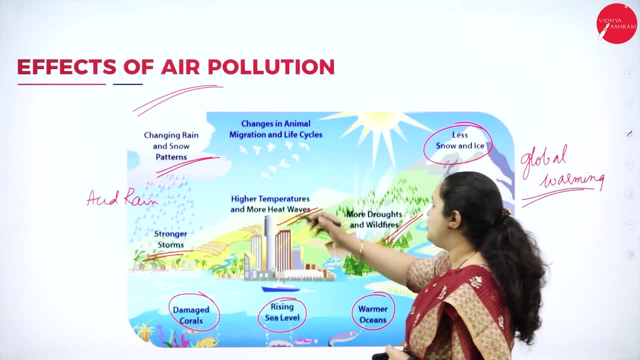 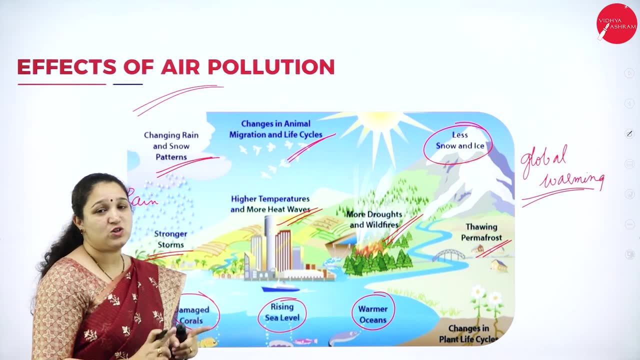 Ok, Thawing the permafrost also can happen. Ok, In animal migration and life cycle. all of this can happen because of the root cause of air pollution. Air pollution is the one which is causing acid rain and global warming, and these two 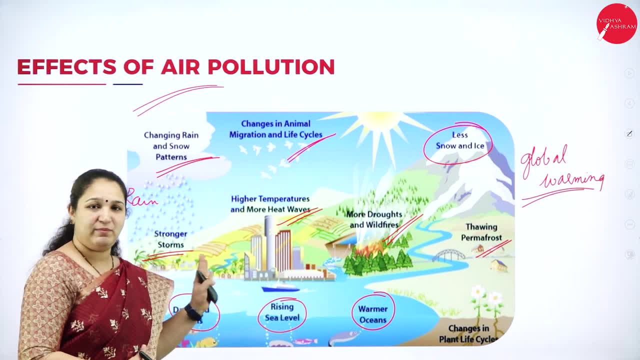 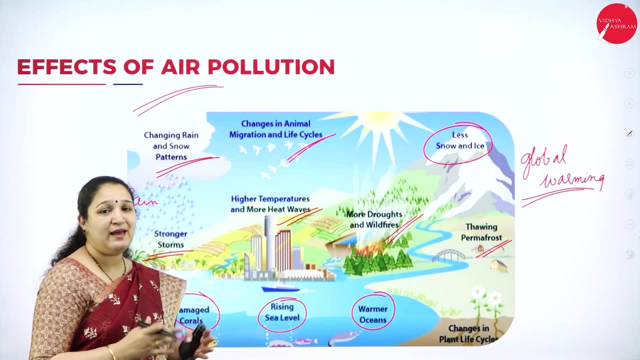 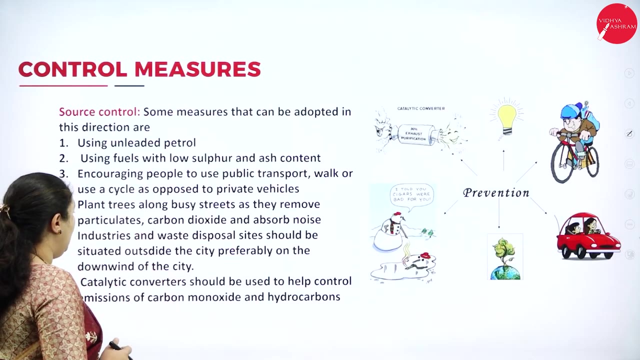 things can give rise to all of these changes in the environment, and all the wild animals, microorganisms, as well as the birds, along with humans, can be affected with air pollution. Next, We can- Ok, We can- have some control measures which we can take to control air pollution. 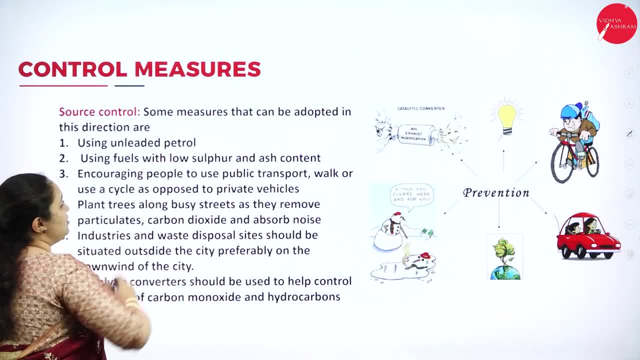 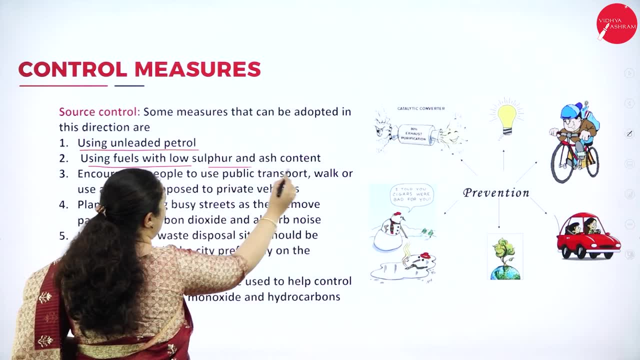 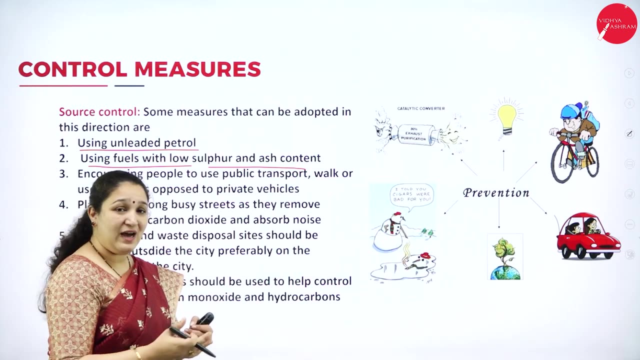 What we can do. First thing is some measures that can be adopted directly are using unleaded petrol, using fuels with low sulphur and ash content. So the fuel which we use, the quality of the fuel, should be really good. only then it should be unleaded. lead should not be there, sulphur should not be there. then we can prevent lead. 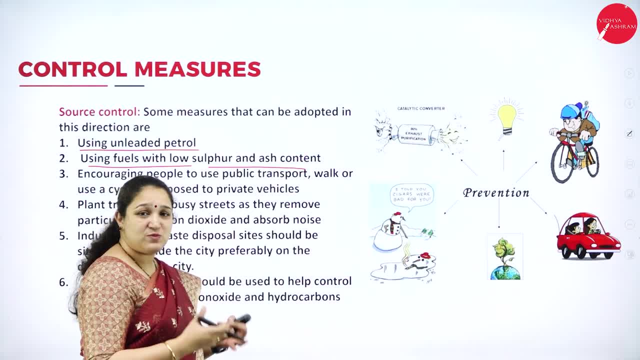 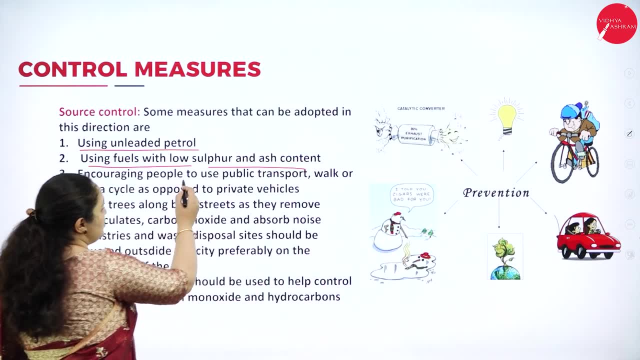 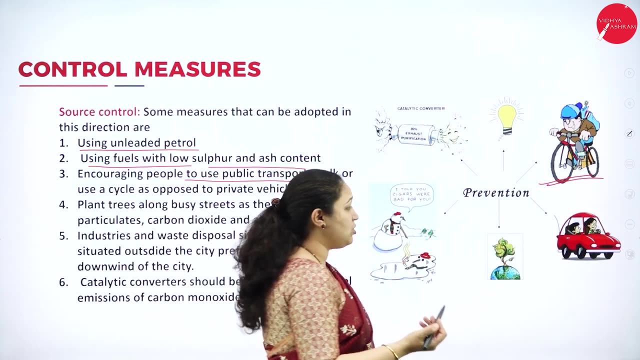 poisoning, As well as the sulphur dioxide which is produced from the vehicles can be reduced, so that acid rain can be reduced, and also encouraging people to use public transport or walk, So some transport, like you know, cycle- can be used or which does not have any pollutants. 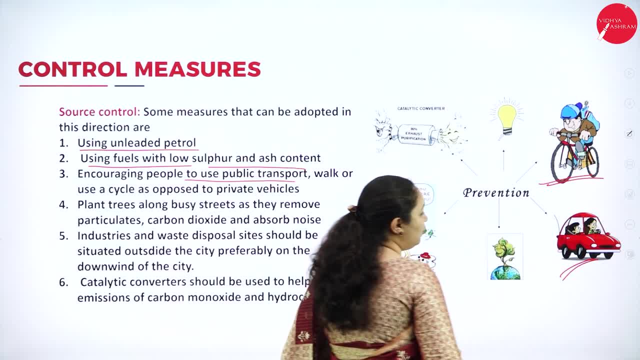 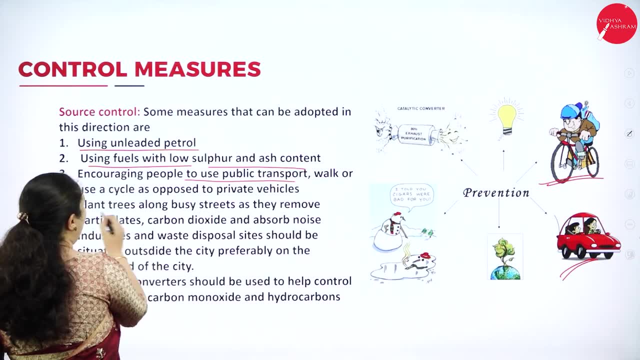 which is coming out from it or we can you know? pooling of the cars can be taking place, or using public transport also can be encouraged. Also, Plant trees along the busy streets so that they can remove the particulates, carbon dioxide and absorb the noise as well. noise pollution also can be reduced. 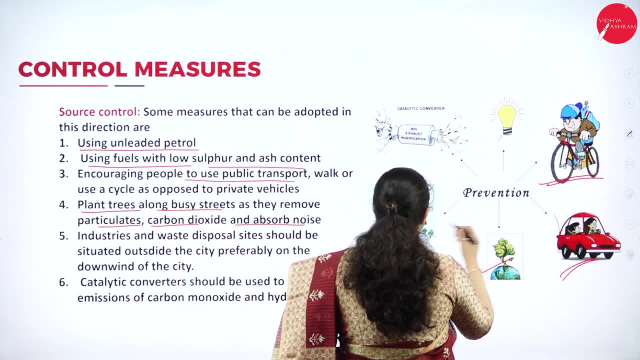 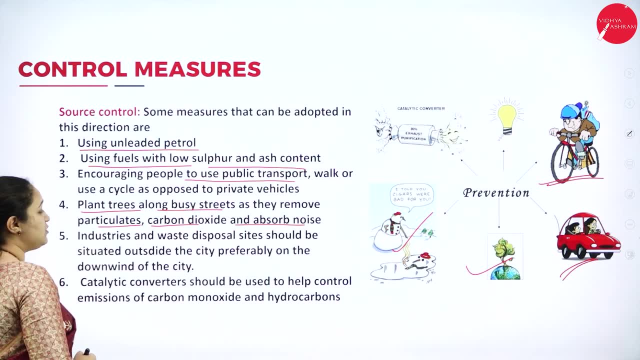 So planting trees again is very, very important. Cigars, again one more cause of air pollution, and industries and the waste disposal site should be situated outside the city, preferably on the downwind of the city. then catalytic converter: This should be used to help control the emission of carbon monoxide. 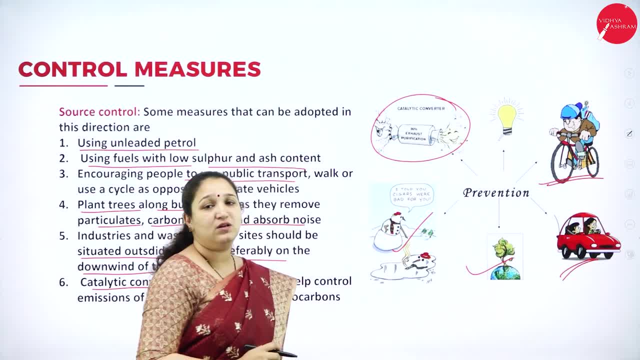 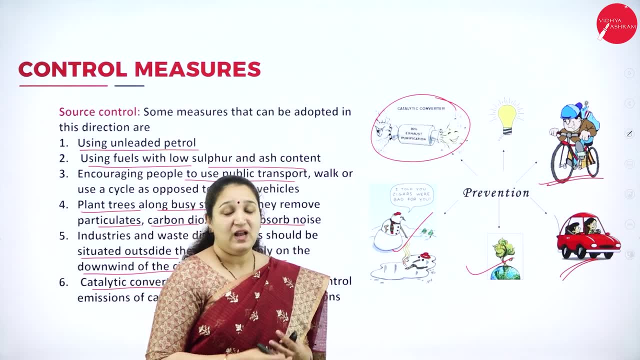 So catalytic converter can be there, can be installed in all the vehicles so that carbon monoxide is reduced and thus, you know, the pollution can be reduced. and also there should be strict action which has to be taken, or the rules which has to be placed on all the 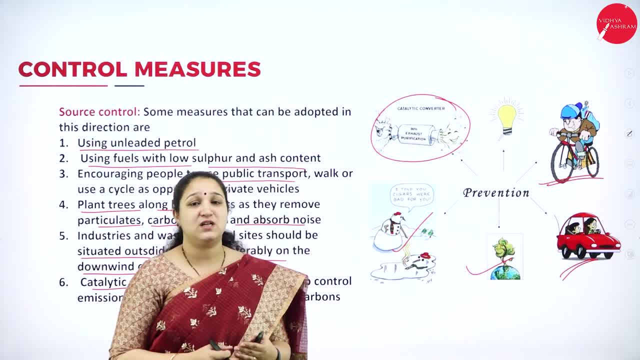 industries so that they can use all the equipments which is required before they leave out the exhaust gases. So if you want to control the air pollution from these industry directly into the air, it has to pass through these equipments so that all of the air pollutants can be neutralized. 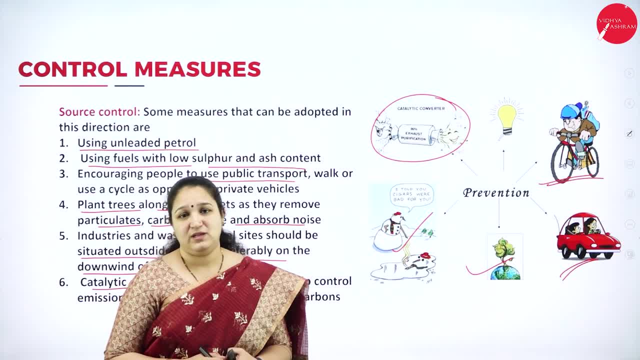 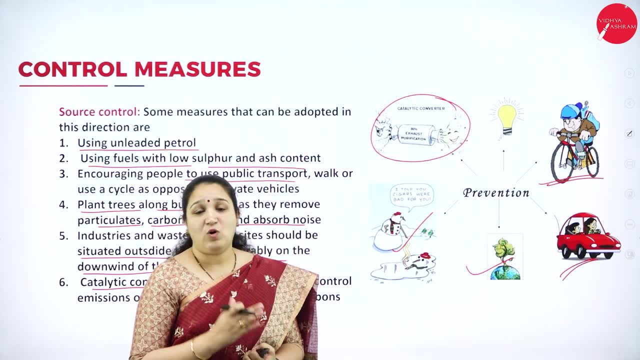 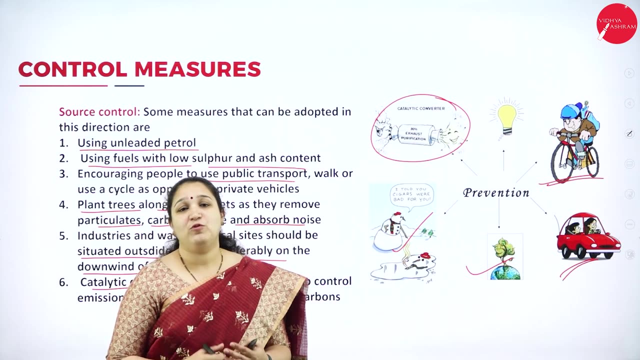 and then it had. it can be left into the environment. So there has to be strict rules on using the equipments and also to control the air pollution and what is the amount of pollution that they are going to cause. All of this has to be taken care by the industries before they leave out any air pollutants. 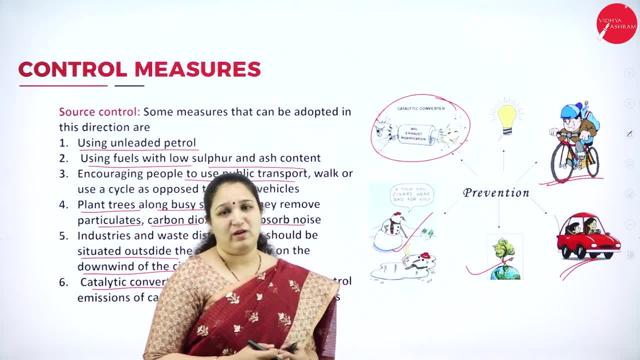 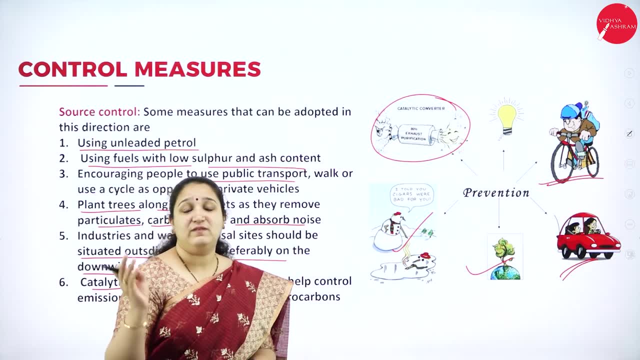 So they will take care of the air pollutants into the environment and spoil the environment. So that's about the air pollution. We have learned about the different types of pollutants. We have learned their causes. We have learned their effects, as well as we have learned about the control measures of. 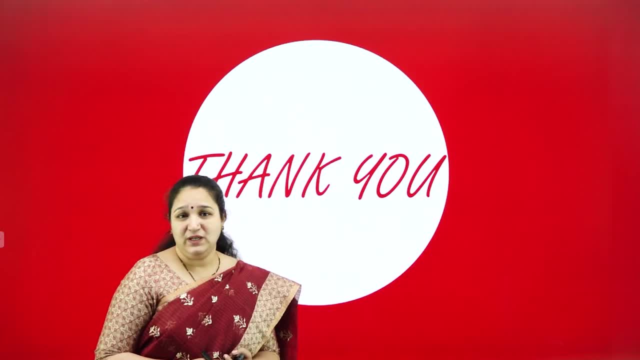 air pollution. So we have to be more responsible to save ourselves and save Mother Earth. So thank you, my dear children, Stay tuned for more updates, Thank you.